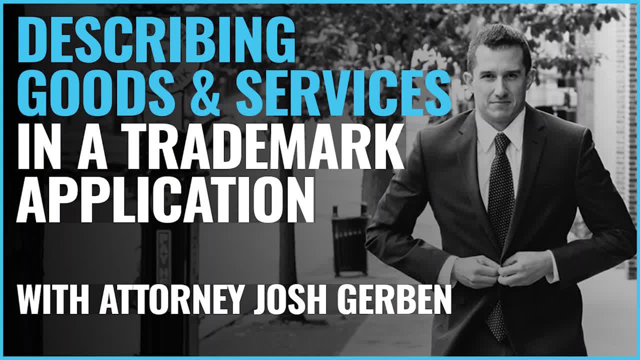 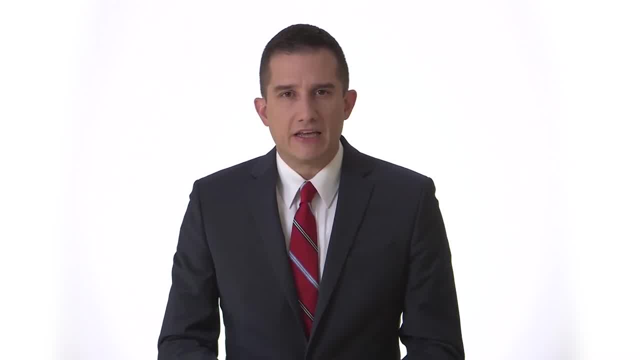 Hi everybody, Trademark Attorney Josh Gerben and I'd like to talk a little bit about how to list your goods and services in a trademark application. So one of the most critical questions in a trademark application is: what are the goods and services associated with your trademark that you would like to protect? 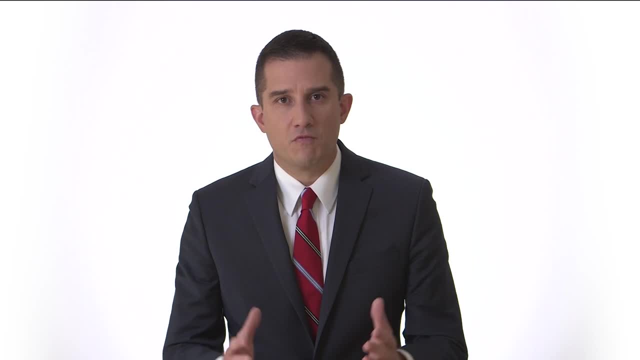 And this question is so critical because it sets the right and scope for your trademark protection. Now, a lot of people will say, oh, I just want to protect my trademark for everything. I don't want anybody else to use my name. That is just not how US trademark law works, though. 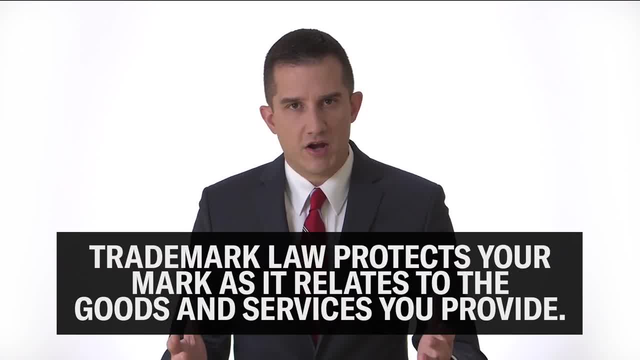 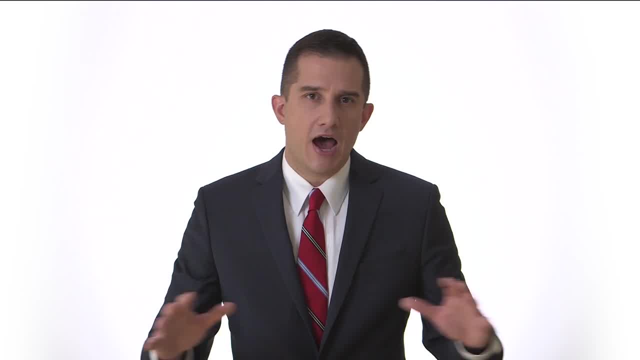 So trademark law protects your name, logo, slogan, your trademark, as it relates to the goods or services that you provide. You can have a monopoly for that, but not for everything. So, for example, you have Delta Airlines and Delta Faucets right. 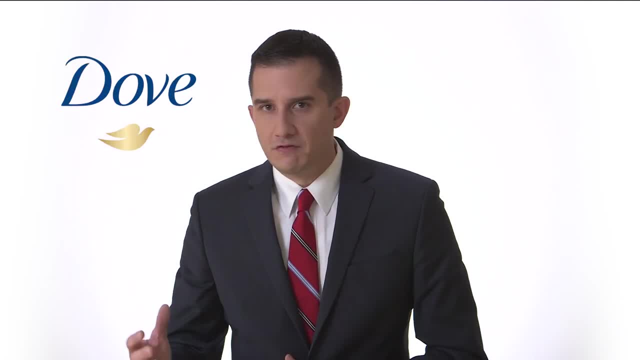 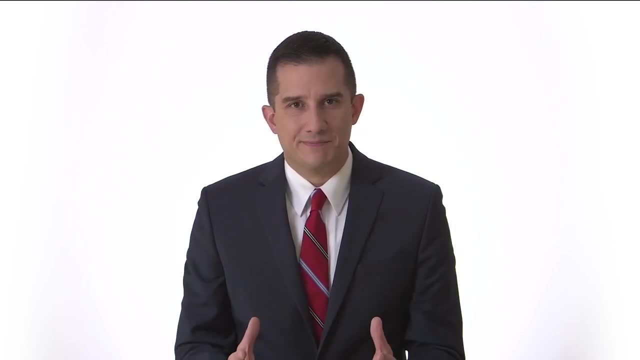 One is an airline company, one's a faucet maker. You have Dove Soap, Dove Chocolate. One's a chocolate maker, one's a soap company. So even these large companies have to share their name, And you may have to share your name as well, but you can expect the rights to extend to whatever you're offering. 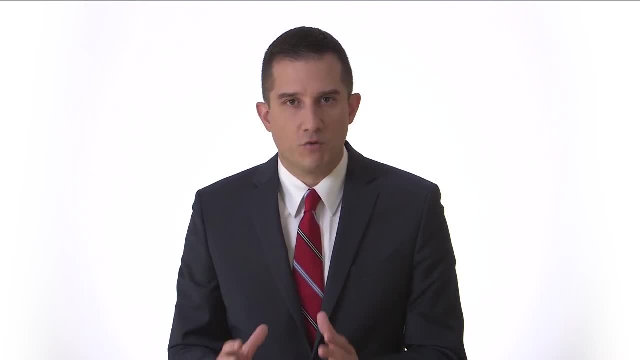 And this is why, when you're drafting that particular language for the trademark application, you have to pay a lot of attention and you have to get it right. So let's take a look at the trademark application itself. Here is the page where you would put in the goods or services that you're offering or plan to use. 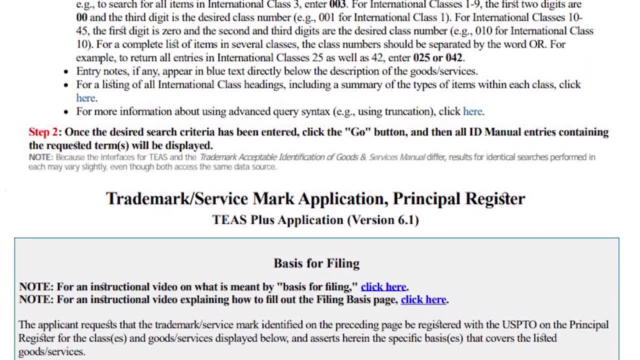 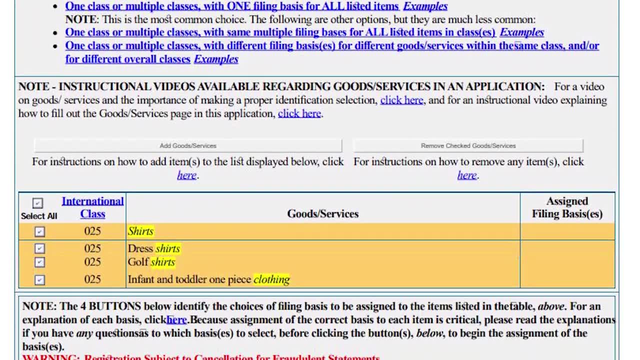 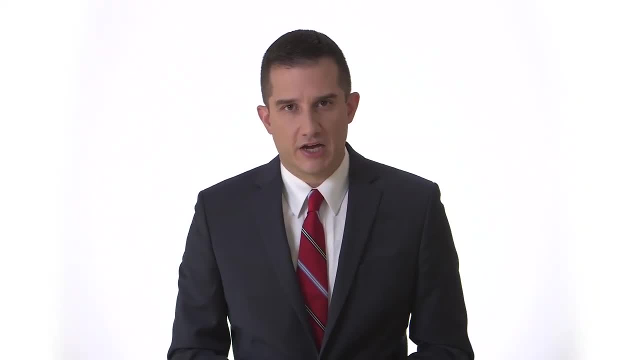 And you can see there's a lot of text here right. The USPTO has a ton of instructions and that's because this is a hyper-technical part of the application that is extremely important to get right. So this can be an incredibly difficult part of a trademark application to get correct. 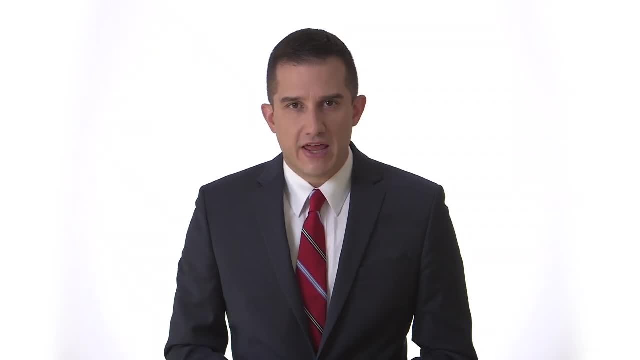 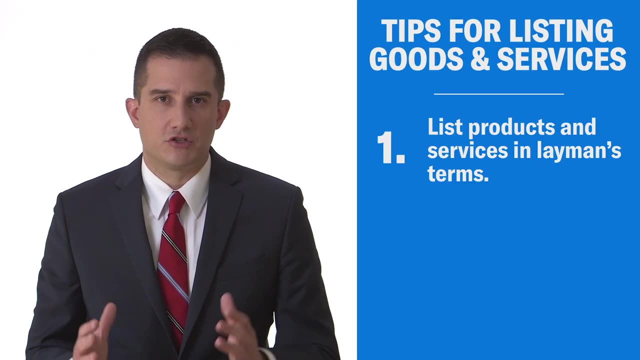 Here are three tips that I use to try to get the best language for any given client into their application. The first is we have to start by listing the products or services you plan to offer, and then we have to list them In layman's terms. 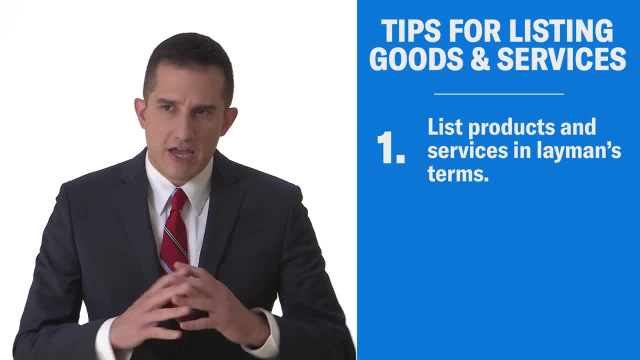 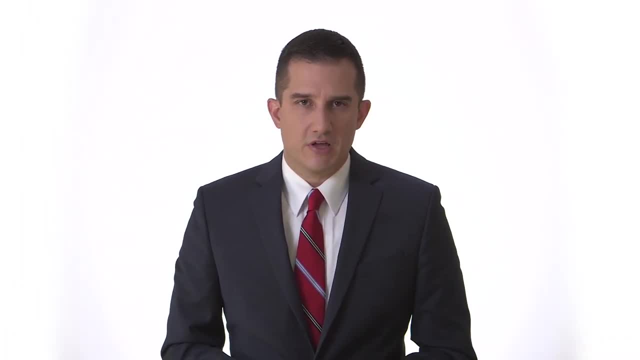 This means stripping out all marketing language, industry lingo, and just being able to write down on a piece of paper what it is you're going to offer. So if it's a clothing brand, are you going to offer shirts and hats. If it's jewelry, will you be offering necklaces and bracelets? 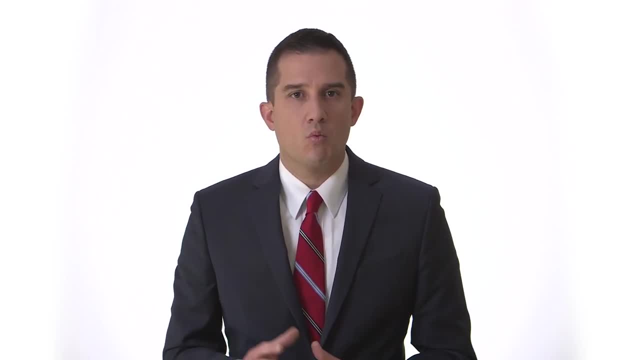 It gets a little bit more complicated. if you're offering a software program, What does the software program do? What are the functionalities of the software program? If you're going to offer a medical service, what kind of medical service? So just being able to write out and understand in layman's terms the goods and services you're going to offer is an extremely important step and surprisingly difficult for a lot of companies to complete. 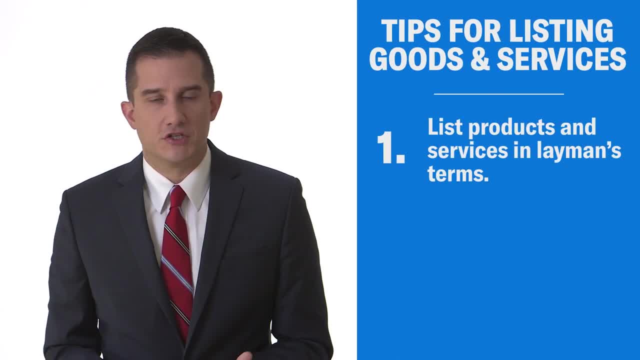 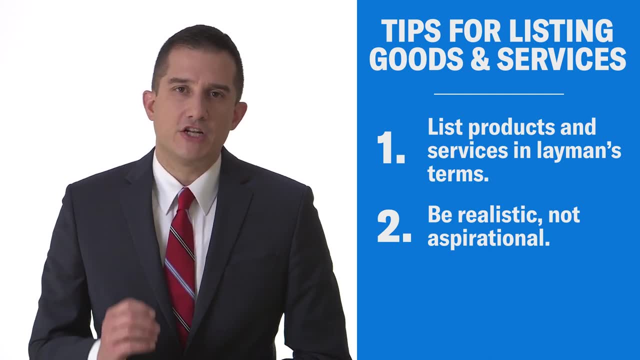 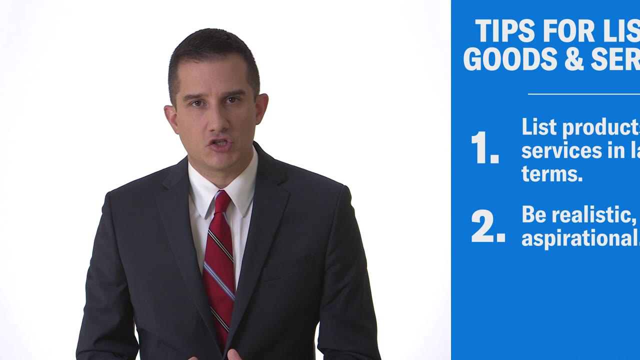 Now the second rule, when thinking about the goods and services you would like to include in a trademark application, is to be realistic and not aspirational. Before a trademark registers, all of the goods and services listed in the application must be actively being sold in commerce. 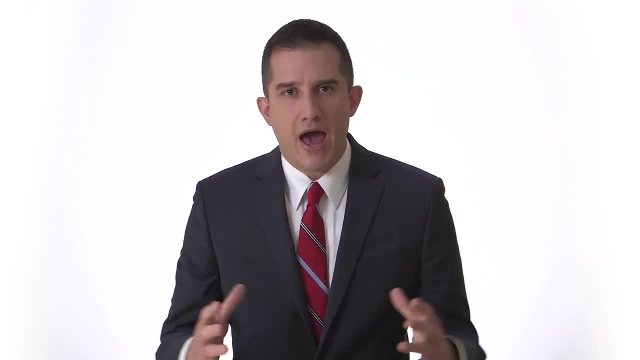 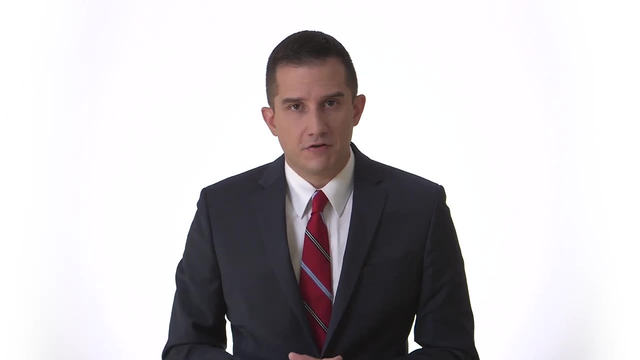 Meaning you actually have to have customers or clients for this stuff. So if you pack your trademark application full of hundreds of products or all these different services that someday you plan to offer, that application cannot mature into a registration until you actually offer everything you've listed. 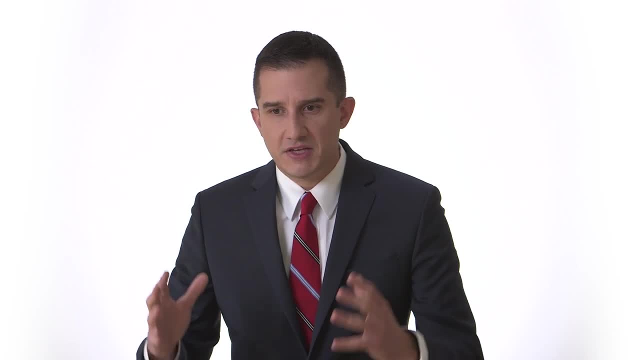 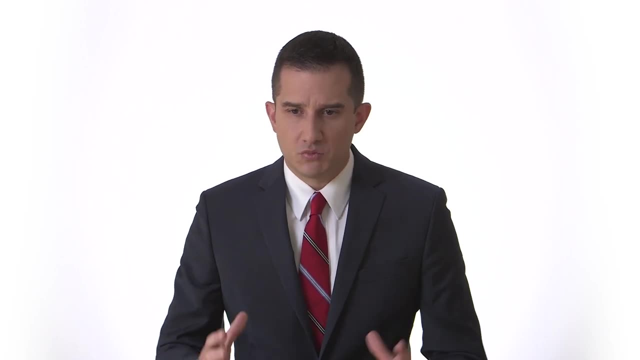 So it just doesn't make sense to come in there and list things that maybe someday you're going to do. You really want to focus on things that are within one to a three year time frame at the most, Because we just don't want an application first off. an application can't sit there for more than really three years. They will just actually cancel out your application if you don't have sales. But you can keep an application active for about three years after the initial filing So you can include things you think are going to be close in the pipeline. But you don't want to be everywhere and just throwing in things because you think someday it's a good idea. 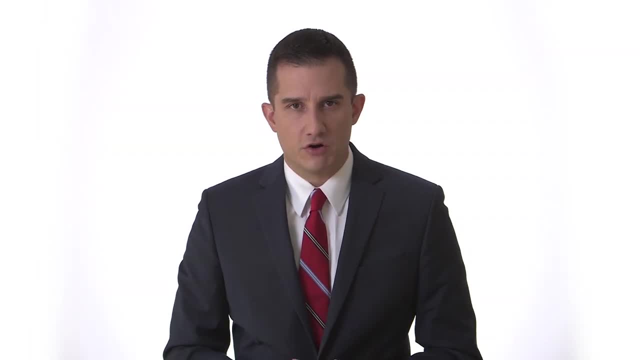 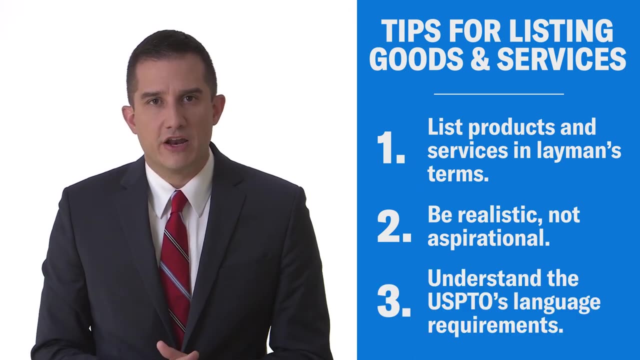 Be very realistic about the goods or services you're going to offer, And my third and final tip is to understand that the USPTO has certain language that it will accept on how you can identify the products or services that you're going to offer. 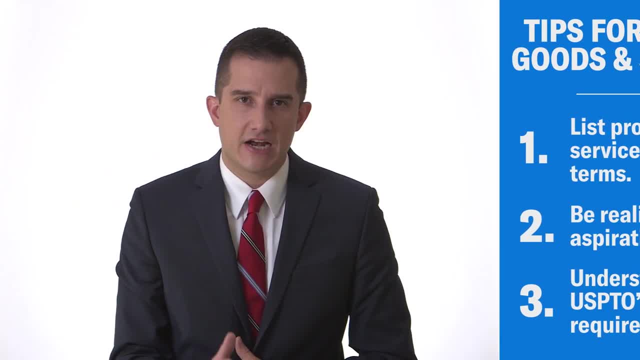 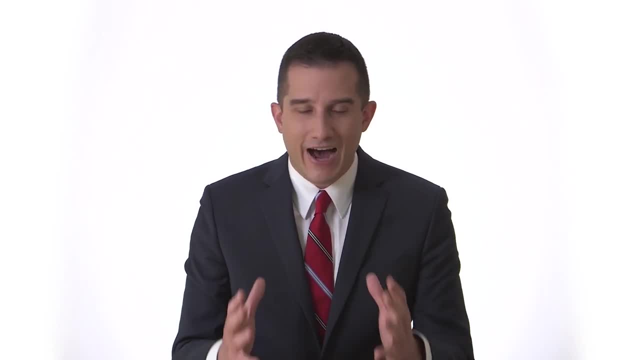 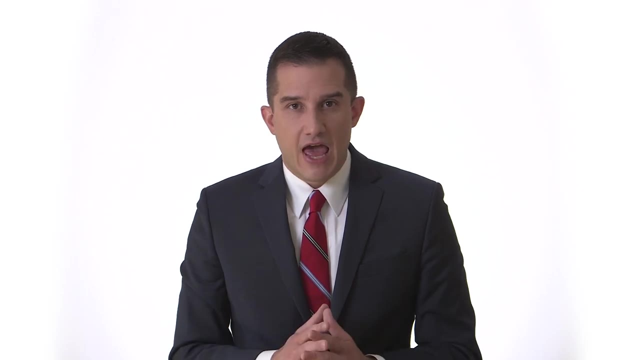 And you can't just make this language up. You have to meet the technical requirements that the USPTO has, So you need to understand what those requirements are, or you need to hire somebody that does Like a trademark attorney. So I do see a lot of clients come to me and they have these marketing statements.